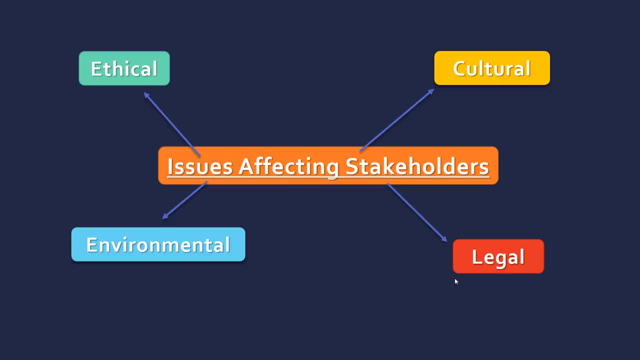 of come up with your own ideas, especially if you're well informed and these sort of things. but there are some talking points you should really know and some theory as well, to do with legal stuff in particular. so make sure you stay tuned till the end, or skip there if you want to. 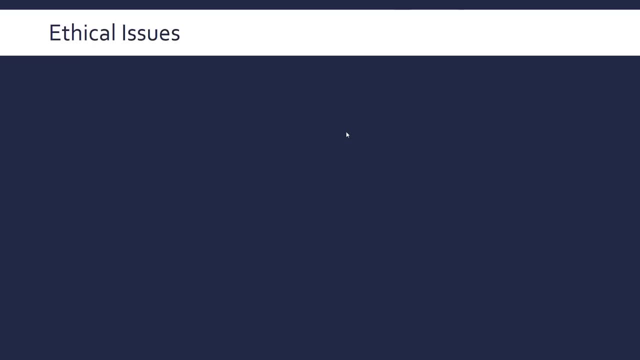 if you're comfortable with the first three. But let's start by looking at some ethical issues first, which is all about whether something is right or wrong. Privacy is a great example of an ethical issue. so to what extent do we have a right to privacy as citizens? There's often a trade-off. 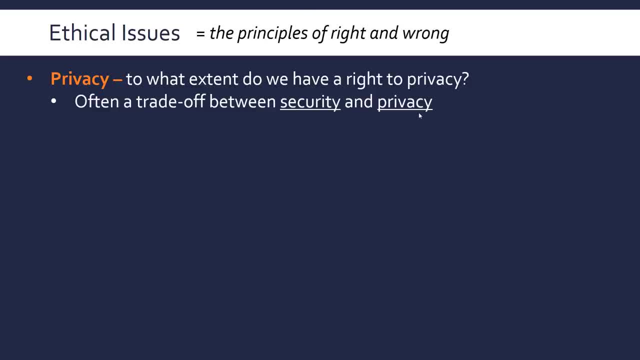 between our security and our privacy, ie protection of our private data. The government need to keep us safe, that's to leave their main business, and to keep us safe, that's to leave their main business role. but that often means that we have to look at personal data in order to, you know, detect crime in. 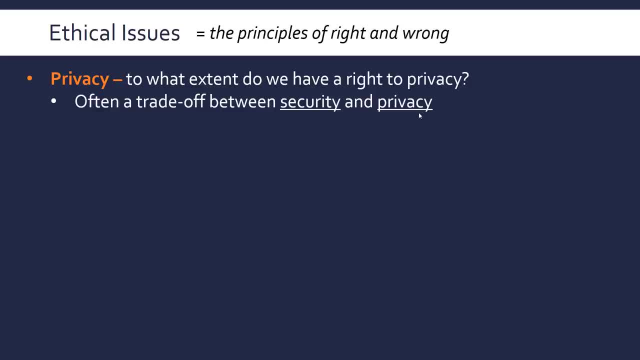 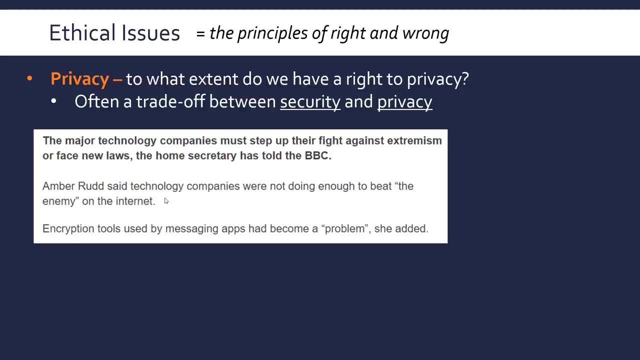 early stage, detect terrorism and so on, which a lot of people don't like. people are very wary of government surveillance, so i could be recording this at any point in time. there'd be loads of examples, and one recently as i'm doing. this is the home secretary's basically told large technology. 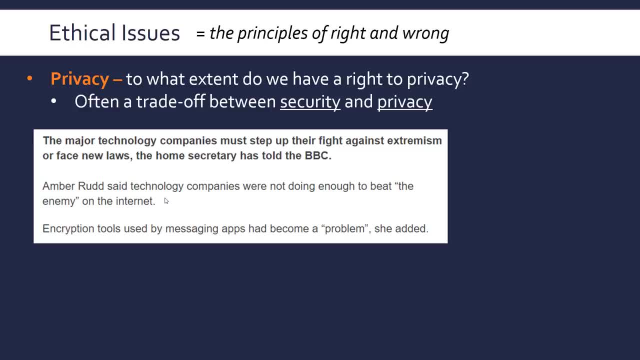 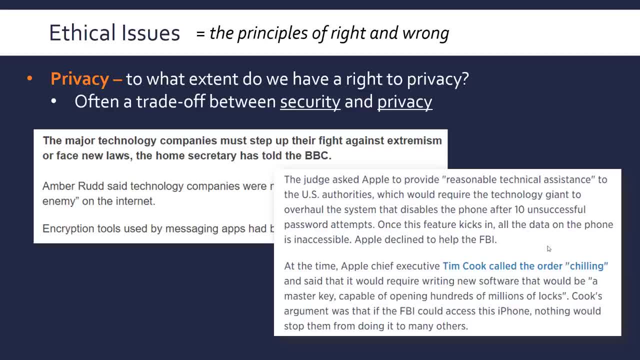 have access to an iphone by basically getting apple to bypass their security system. apple refused because they thought it would undermine their system and it set a bad precedent, even if this was a one-off case. eventually the fbi got in anyway, so that kind of suggested that something. 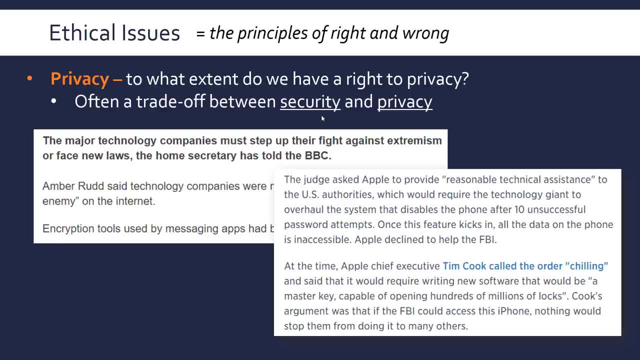 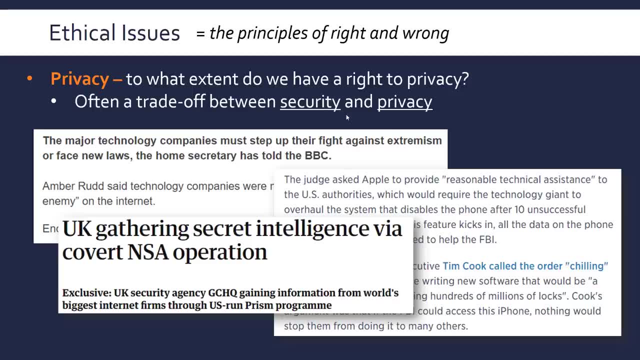 wasn't quite up with apple security system. maybe it was weaker than it should have been. and on a larger scale you have mass surveillance by the nsa and gchq of their citizens. clearly they'd say it's for security, but most people feel kind of uncomfortable. 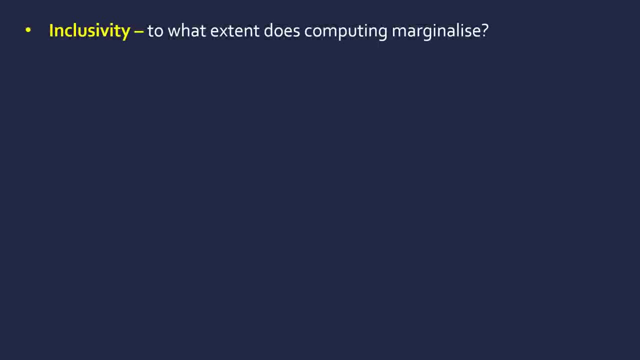 by that idea. there are tons of ethical issues, clearly, but a second good one is all about inclusivity, making sure technology is inclusive. so to what extent does computing marginalize people? so as technology becomes more prevalent in our society, it may negatively impact people who can't. 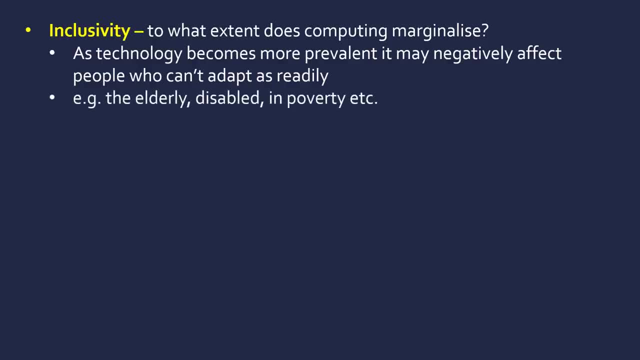 adapt as readily to this change. so people like the elderly people are disabled people who are in poverty. so certain countries that just don't have the infrastructure, don't have the money to spend on technology, they may get left behind in the world economy and on a kind of individual level. 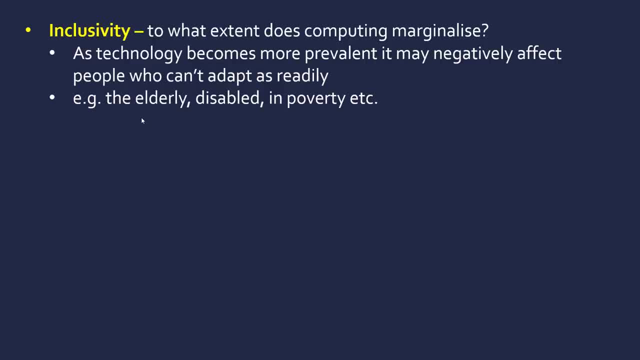 people who are perhaps not used to this technology may not be able to adapt as the world around them does. and finally, professionalism is something you could talk about. so does computing help in a work context? does it make people work better? does it make people work more professionally and just in? 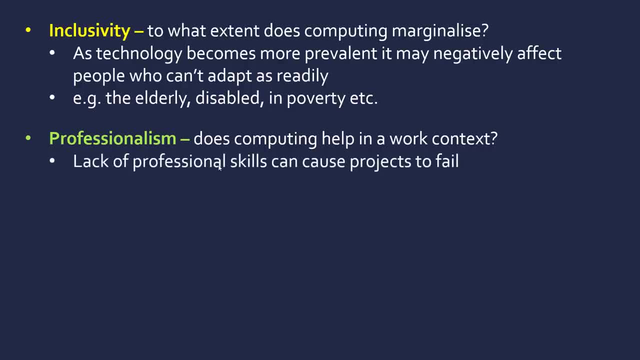 general lack of professional skills can cause projects to fail. so these skills being like communication, teamwork, etc. there's often a module in a computer science degree just for professional skill development, and so a lack of ethical training or standards in the kind of computer science community can lead to. 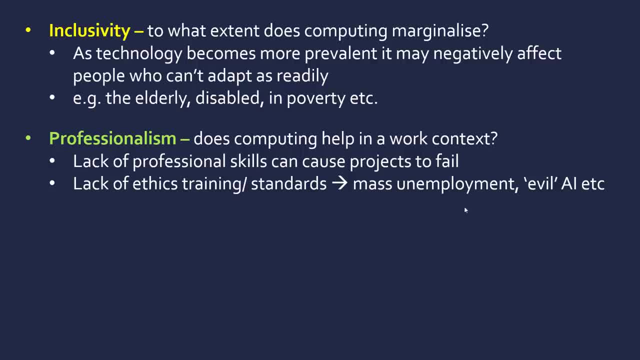 things which may spiral out of control. so a very drastic step here. but if people don't consider the ethical issues at a very early stage, you may end up with things like mass unemployment through just computers taking over most low skilled jobs and, in a very drastic example, maybe AI which is evil. 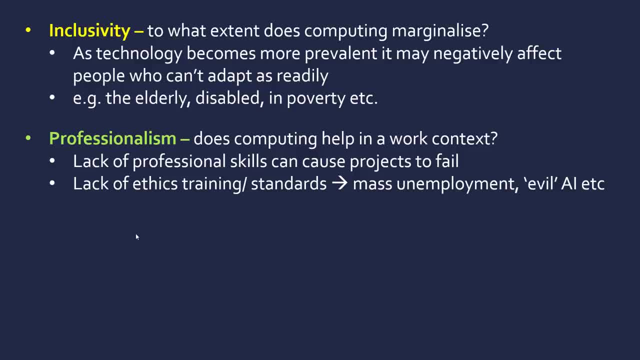 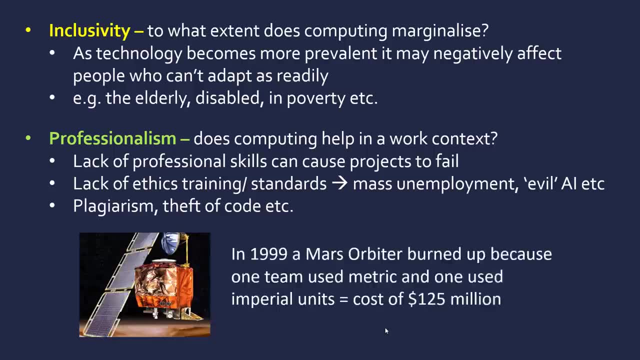 if people don't consider the small ethical issues, they can kind of snowball. and another example which is perhaps more related to ethics is things like plagiarism, the theft of code. an example of a project which went badly due to a lack of professional skills is this NASA orbiter, which 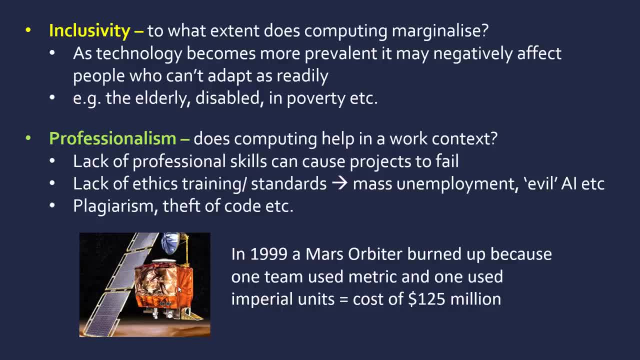 is a project that went badly due to a lack of professional skills. is this NASA orbiter, which is a project that went badly due to a lack of professional skills? is this NASA orbiter, which blew up in 1999 because one team on the project used metric units. one team unit used imperial? 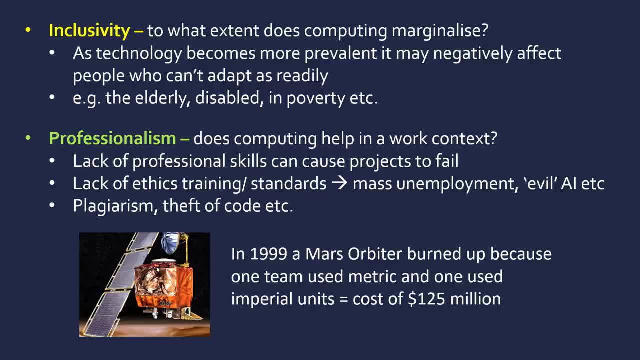 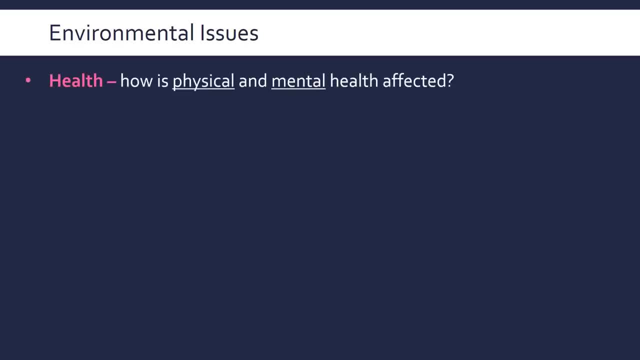 units and unfortunately no one died. this was an unmanned orbiter, but it cost 125 million dollars, so a huge project down the drain. a second category we can look at are environmental issues related to computing. so first of all, health. so how is our physical and mental health affected? 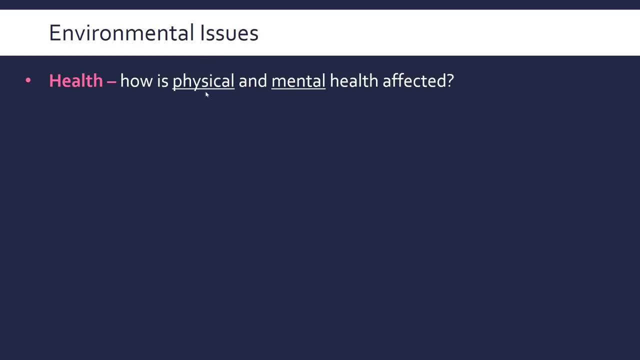 both really important. up until maybe five, ten years ago only physical health would be really considered, but now mental health is much more important in the kind of public perspective. so you may. the initial kind of reaction to that is: perhaps technology negatively affects this, but it actually can improve it on a small level, obviously in the 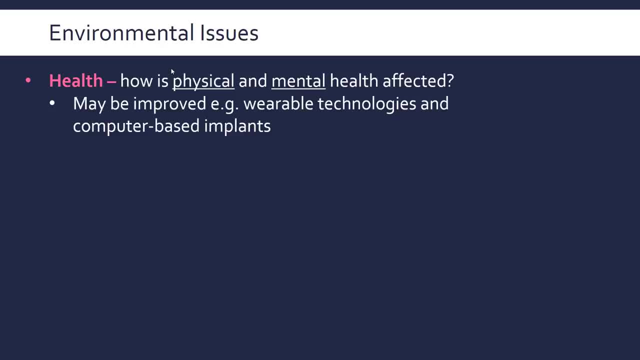 medical profession. technology has made a huge difference, but we're talking kind of on an individual level. so perhaps through wearable technologies like smart watches or fitbits allow people to have a better understanding of their body and so how they can improve their health. and in the future, maybe computer-based implants where little devices are inserted into our bodies as 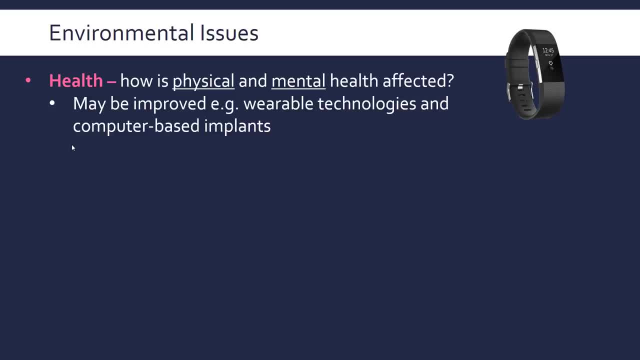 implants and they maybe can help regulate the body and so on. but that obviously causes its own issues that you could talk for ages about in terms of how it negatively affects- i guess it's stating the obvious a bit- but mental health maybe. social media is not healthy, especially for younger children, and 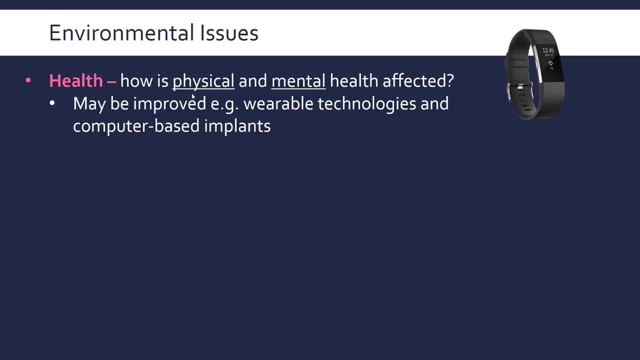 physical health. perhaps in general, people using technology- like, again, young children- can make them less active than they would be otherwise. energy use is an obvious environmental issue. so as you try and get more and more computing power, both individually on a single process and collectively in just loads of devices worldwide, you're going to have a lot more. 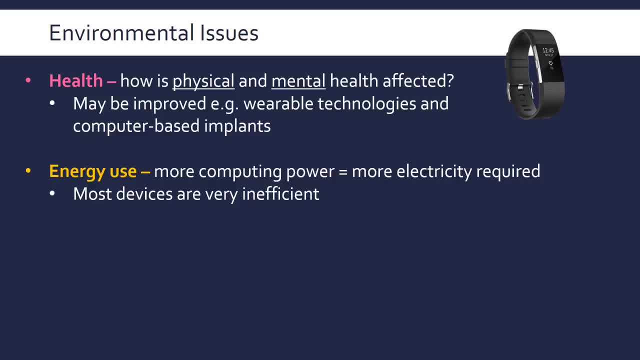 energy use is an obvious environmental issue. so as you try and get more and more computing power, both individually on a single process and collectively in just loads of devices worldwide, you also need more and more electricity. most of this electricity is coming from non-renewable resources, so you know that's a whole environmental issue and, generally speaking, most. 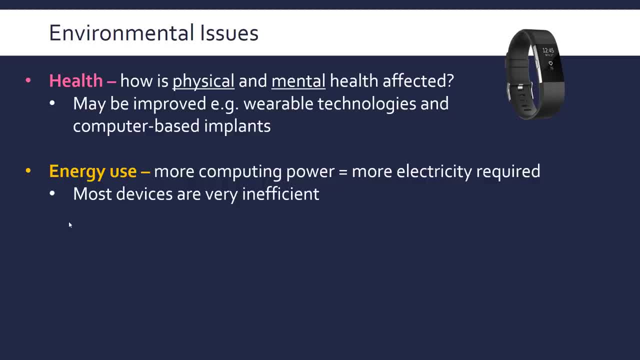 devices are very inefficient. maybe your process is only running at one, maybe ten percent of its capacity if you've got a multi-core processor, so you're wasting so much power. if the computer's going to be on all the time, you just maybe won't be using it. so inefficiency causes way more energy. 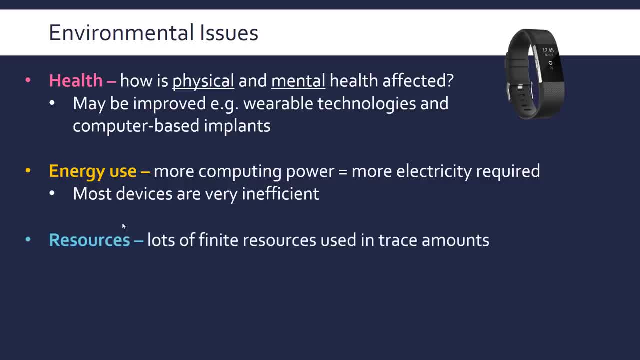 use than it should do. maybe a less obvious issue is resource depletion in terms of computers specifically. not just about non-renewable resources, but not just about non-renewable resources, but lots of these finite resources are used in trace amounts of tiny amounts in our devices, things like. 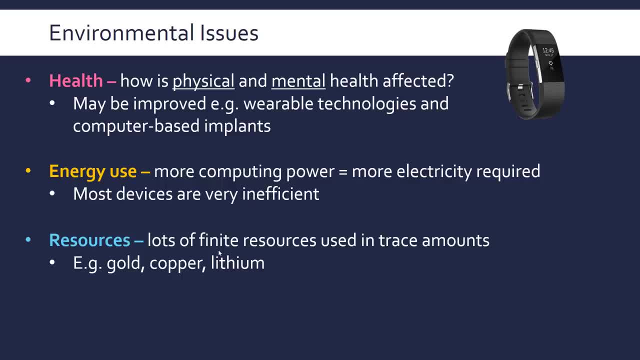 gold, copper, lithium. they're used in very small amounts but collectively in terms of all the output of all iphones. whatever they're used in huge amounts overall and because they're used in such small amounts they're very hard to extract when you perhaps recycle them, and people don't even. 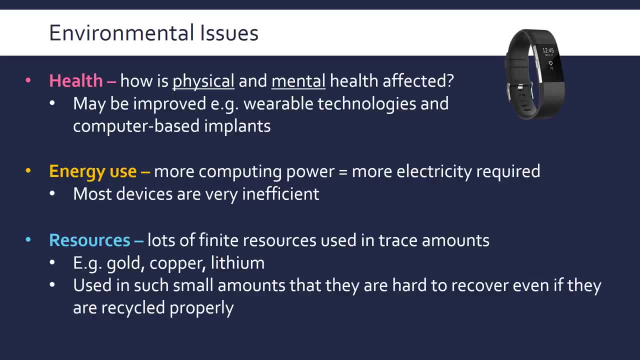 recycle them anyway, perhaps. but even if you could recycle, it's very difficult to get a tiny bit of gold back. in fact it's not really worthwhile. but as you add it all up, you're then losing so much gold to landfill, for example. look at cultural issues then, which is a very broad and kind of vague. 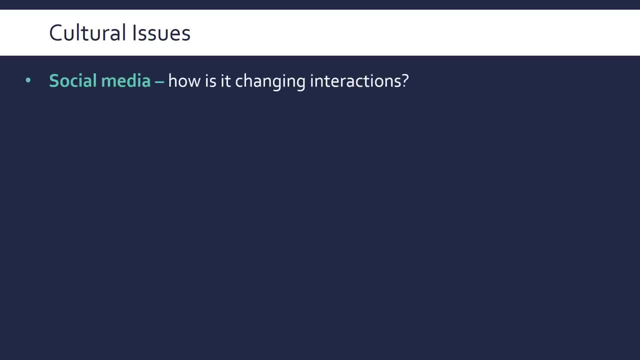 category to be fair. but you know, social media could be a good thing to talk about. how is it changing interactions in a culture that uses lots of social media? perhaps it's better at holding businesses or politicians accountable. it's a good way of spreading information, both in a good and bad way. 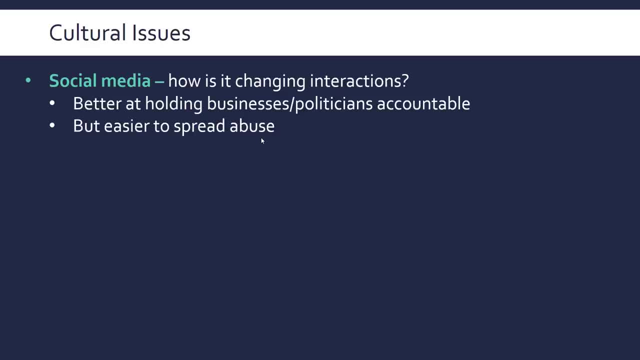 in terms of like spreading abuse, trolling and so on. social media can definitely negatively impact a whole culture and, as i say, it can be used to influence opinions, both in a good or bad way, depending on your context, but even from outside sources, like the russian hacking in the us election that was mostly through a misinformation. 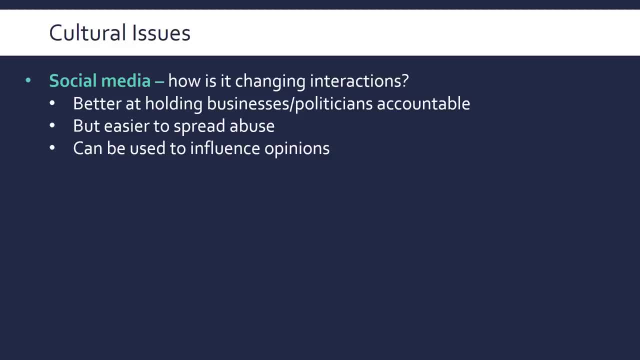 campaign on social media. so you've got to be very careful and it can definitely change your culture and employment. you can put employment in lots of different categories of these kind of general issues, but this is about how will technology change the job market in particular, how will the lower skill workers react? how is that going to change the setup we have in our culture? 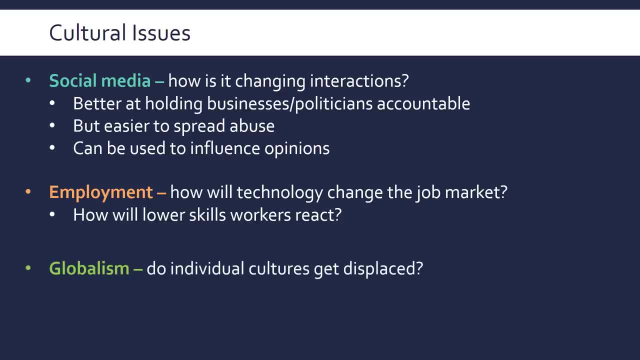 another similar theme. globalism is something you can talk about with cultural issues. as the world becomes more and more connected and so much is shared online, do individual cultures and traditions get displaced by just a generic worldwide community? so globalism is a bit of a toxic term politically, but there are loads of benefits and some disadvantages to globalism. 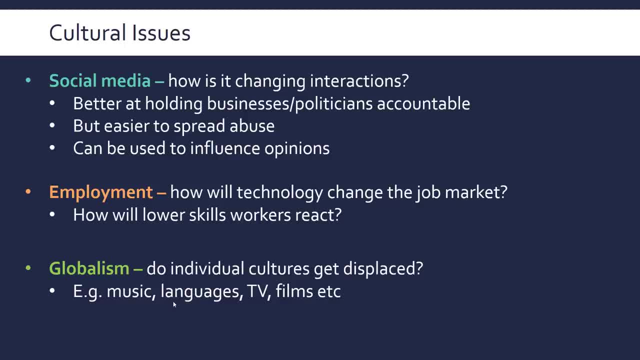 everyone kind of would concede that. um, so take languages, for example, because that's very relevant to computer science. english is the main language for computer science. to program your programming in english, regardless of your native language, pretty much, which isn't totally fair, but is somewhat so. pretty much, if you want to work on technology, regardless of where you live, you kind of need to. 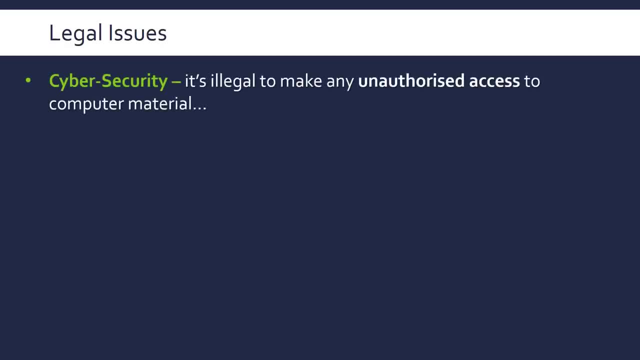 learn english to get far. so focusing on some legal issues- and cyber security is probably the main, most contemporary one, certainly. so it's illegal to make any unauthorized access to computer material if you're going to commit further crimes such as blackmail. so if you collect the data, perhaps 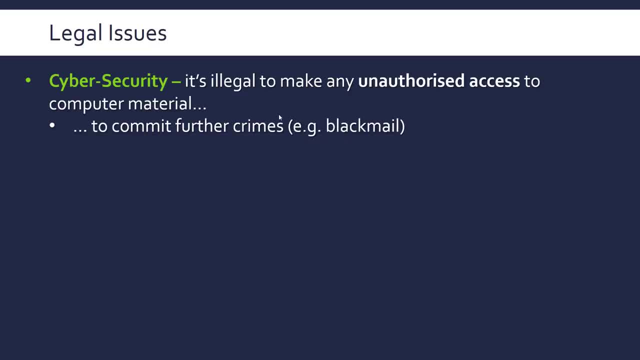 with spyware and then blackmail someone, that is gonna. that's breaking the law clearly and also generically to impair just the computer's operation, so through viruses, hacking and so on. so this is going to be a bit of a wait and see whether or not this is going to be legal. um, it's going to be. 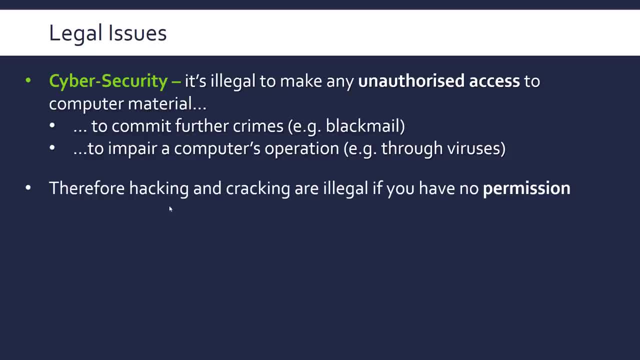 legal if you're not already on the internet. so if you're still on the internet, then of course, if you're doing it as part of a testing team and you've got permission to actually try and break a system, then that's not going to be illegal hacking. cracking may have covered this briefly. 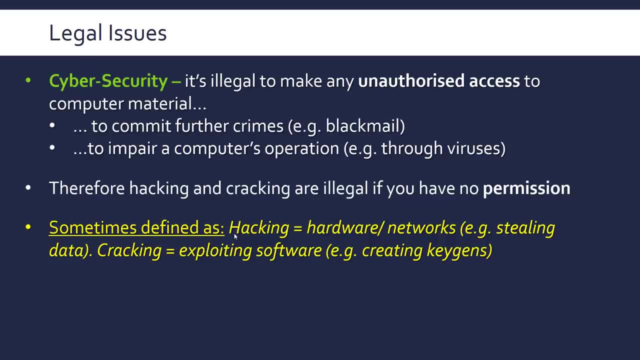 in the security video, but they're kind of loose terms. hacking, at least in my mind, is more about hardware and networks- so getting into a system to steal data perhaps- and whereas cracky is more about software, so exploiting some issues in software like a back door or something. and 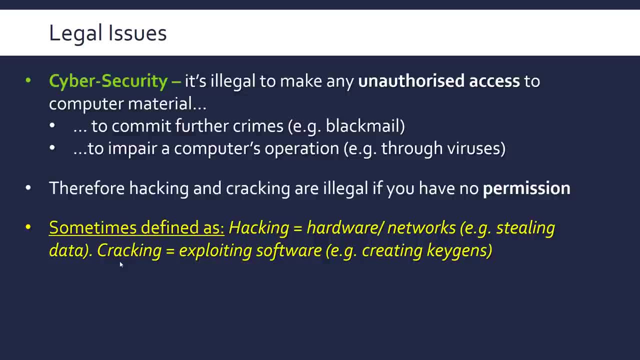 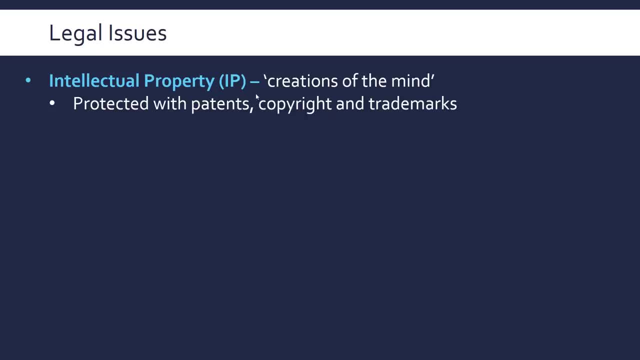 license. so that's, at least in my mind, what cracking is. Maybe a less clear-cut legal issue is intellectual property rights, and the very vague legal definition is that they're creations of the mind. that's what IP is: creations of the mind. so things like inventions, a new algorithm, a new piece of software and 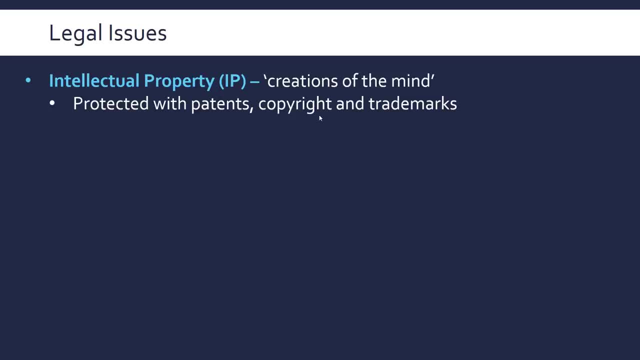 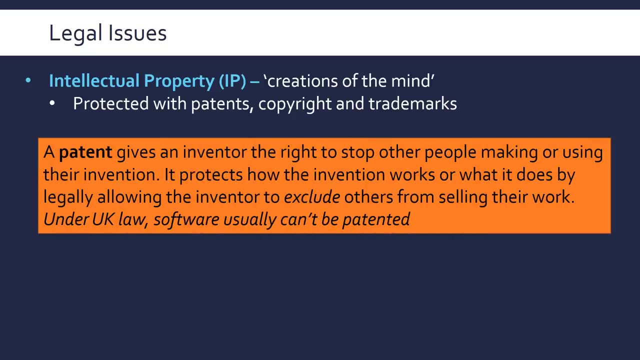 you can protect from the patents, copyright and trademark. so maybe patents and copyright are more for the actual product itself, whereas trademarks are more for marketing the product with the brand. A patent is a legal document. I suppose it gives an inventor the right to stop other people making or using. 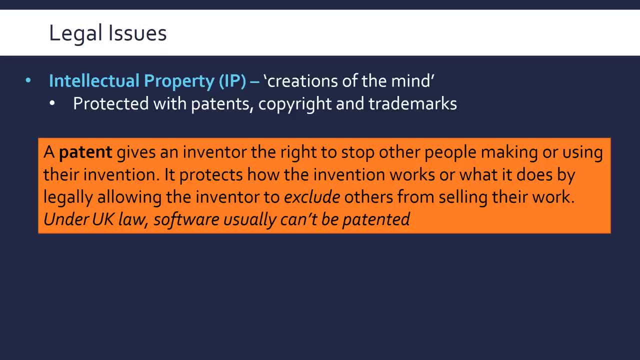 their invention and you have to apply to it. so it's something the government will give you and it protects how the invention works or what it does, by allowing the inventor to exclude others from selling their work. and actually under UK law, software usually can't be patented and copyright is just the legal 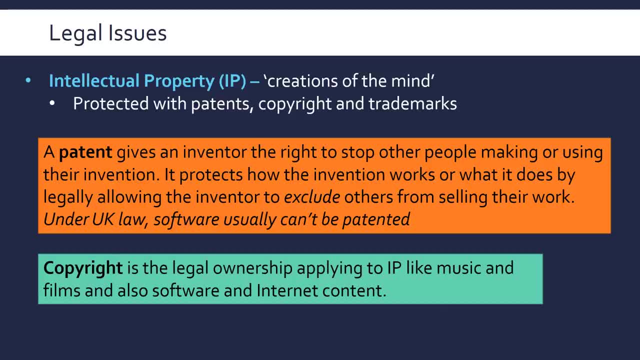 ownership. that applies to intellectual property and you don't have to apply to get copyright. you just have copyright by being the author, whereas you have to actually get a patent from the government, and copyright is all about permission. so if they don't give you permission to distribute a film, it's going to be illegal if you give it to someone else. 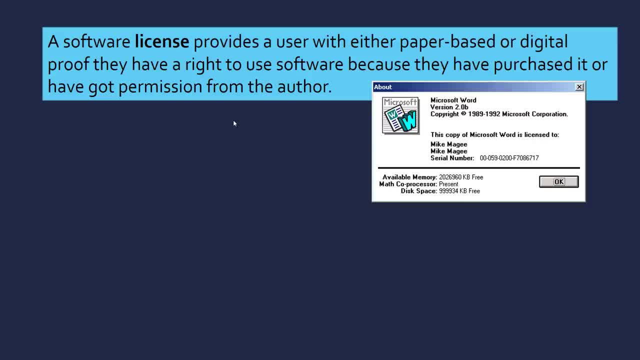 for free Licensing is all about kind of proving you haven't stolen some copyrighted software. so a software license is either paper-based or digital and it basically shows that you have a right to use software because you have purchased it or have got permission from the author, which is kind of the same. 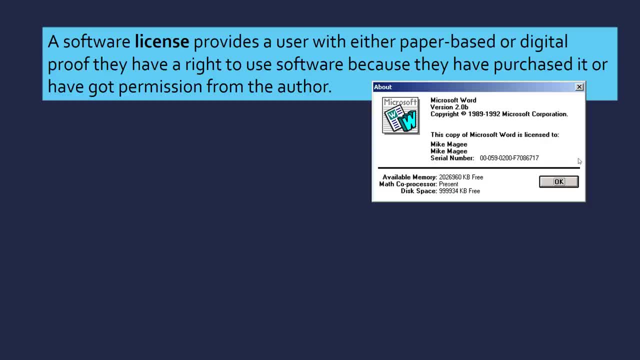 thing, I suppose, but they can maybe give it to you for free. so you often have software. a license maybe has a serial number you have to enter to download software and it basically will have your name and other details showing you you're allowed to use it. 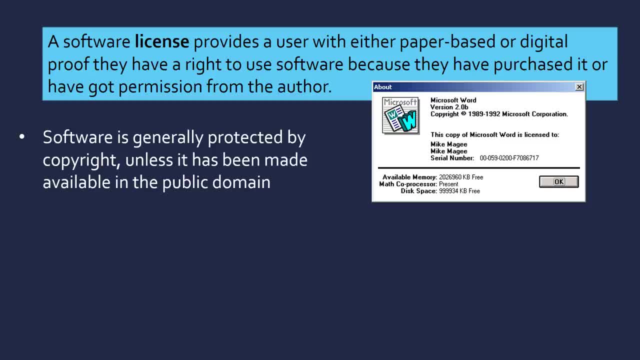 So generally software is protected by copyright unless you've explicitly put it into a public domain. but even if some software is free, you still may have to agree to a software license and in fact you do in most cases still have to kind of agree to terms and conditions, usually at a minimum saying you can't then sell it on to. 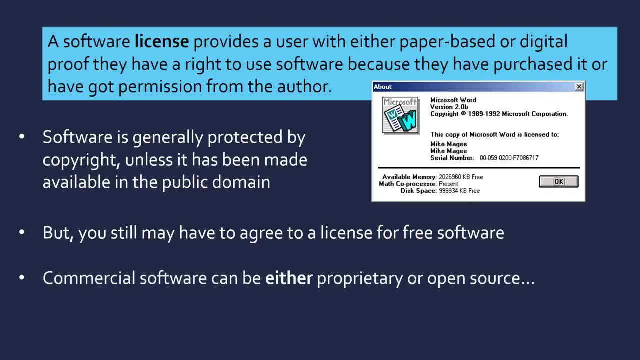 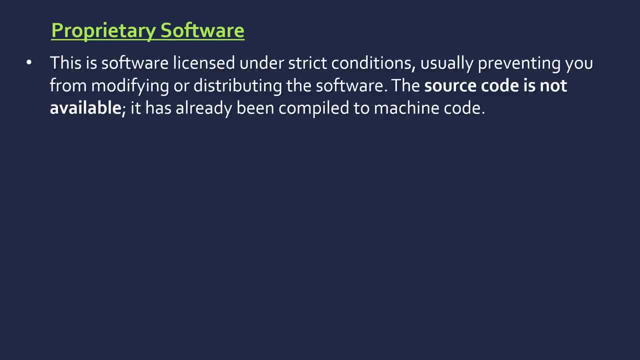 someone else if you've got it for free yourself and as a category, commercial software- ie software that's sold- can either be proprietary or open source. so, first of all, proprietary software is software licensed under very strict conditions, usually preventing you from modifying or distributing the software yourself and, crucially, the software. 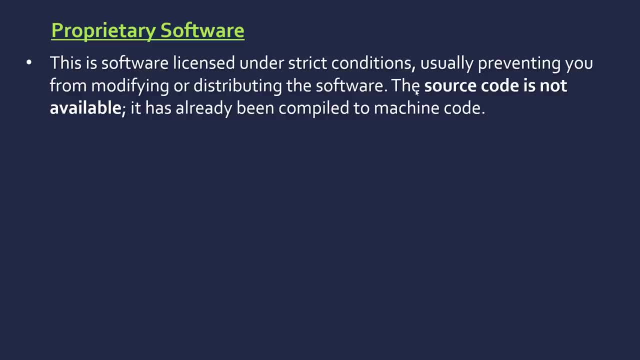 and, crucially, the source code, I should say, is not available to you as the user. it's already been compiled to machine code, so a compiler is taking the source code and making a machine code. the source code is not kind of shipped with a software, so with proprietary software, basically the only thing you can do is use it.